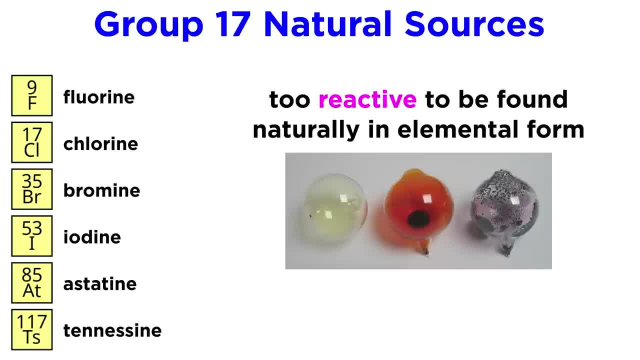 Where can these elements be found? They are actually too reactive to be found naturally in elemental form, but they can be found in a variety of compounds and separated by electrolysis or oxidation. Fluorine is present in ores like fluorite, which is widespread. 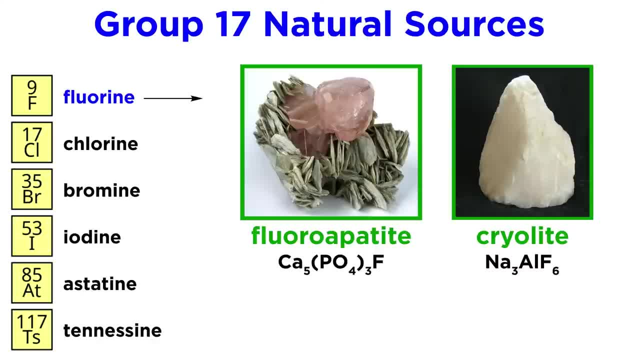 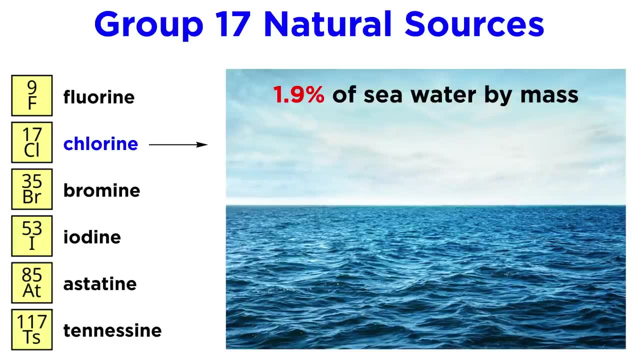 with the largest deposits located in South Africa, as well as fluoroapatite and cryolite, the latter of which is found mainly in the United States, Canada and Russia. Chlorine makes up 1.9% of seawater by mass due to its salinity. 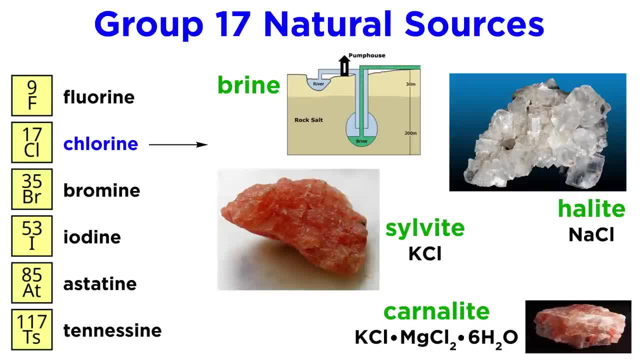 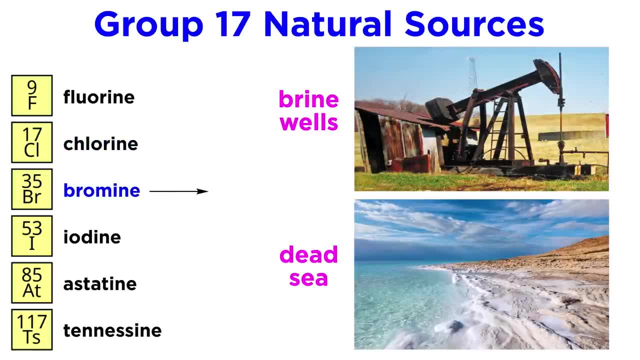 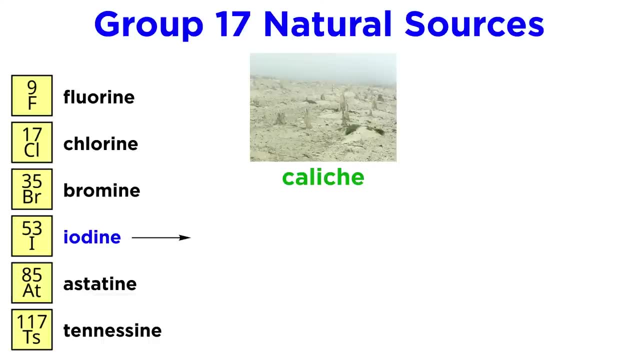 and is also found in underground brine and deposits of halite, sylvite and carnelite. Bromine is found in brine wells and the water of the Dead Sea. Iodine is present in certain salts found in Chile in a layer of soil called caliche, as well as underground brines, saline. 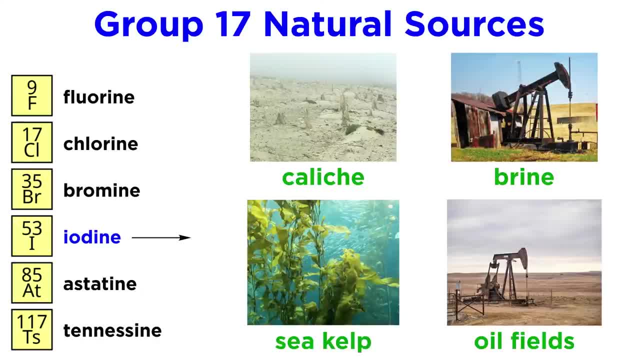 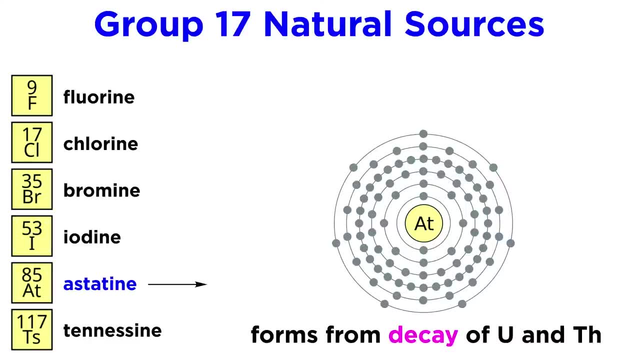 sea kelp and oil fields of Japan and the United States. Astatine is formed from the decay of uranium and thorium in certain ores. It has 32 isotopes, the most stable of which has a half-life of about eight hours. 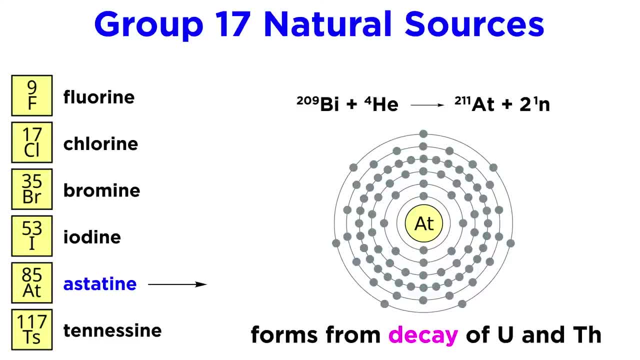 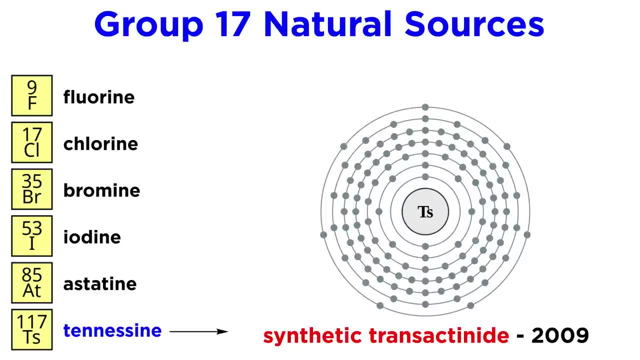 It can also be made synthetically by alpha bombardment of bismuth-209.. Tennessine is another strictly synthetic transactinide element, first made in 2009,, and it's most likely to be found in the United States. It is also found in the United States. 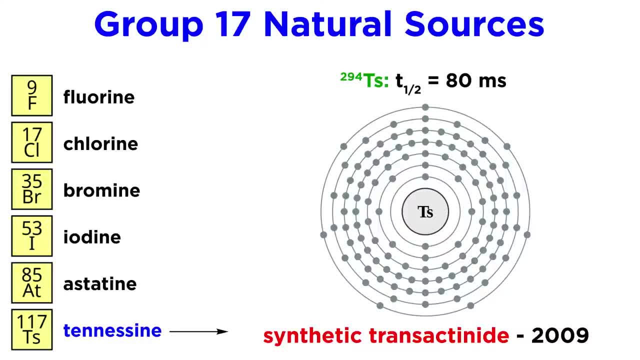 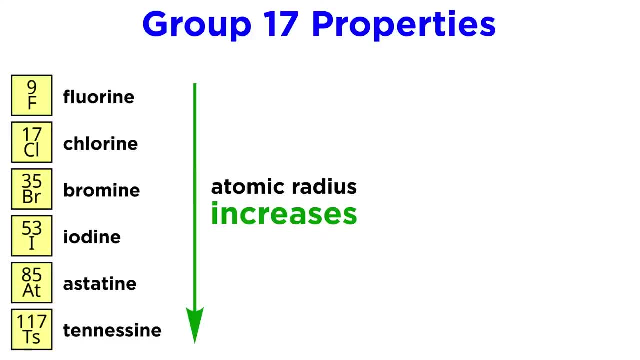 Its most stable isotope has a half-life of 80 milliseconds. Now let's talk about properties. Of course, we know that atomic radius increases going down the group and this has an impact on their physical properties. Fluorine is a yellow diatomic. 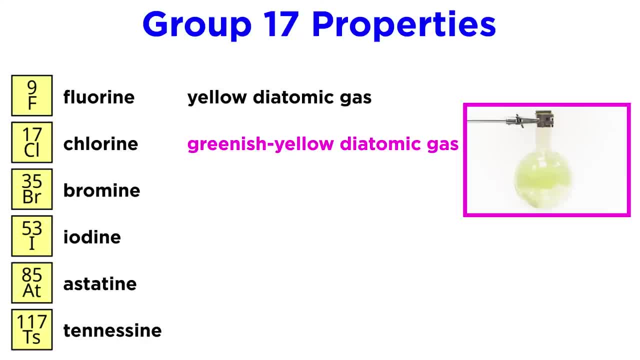 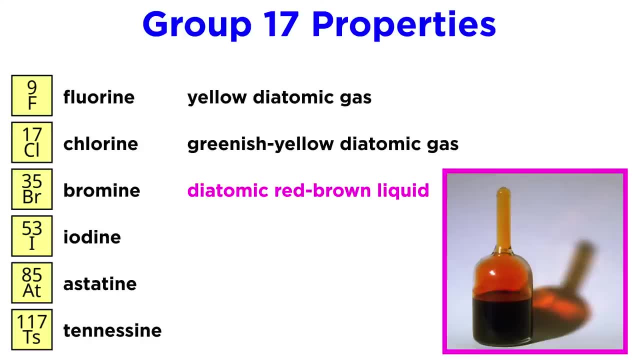 gas Chlorine is a greenish-yellow diatomic gas. Bromine is also diatomic, but it is a red-brown liquid at room temperature with a high vapor pressure. Quite interestingly, this characteristic applies only to bromine and mercury. all other elements in their most stable allotrope are either: 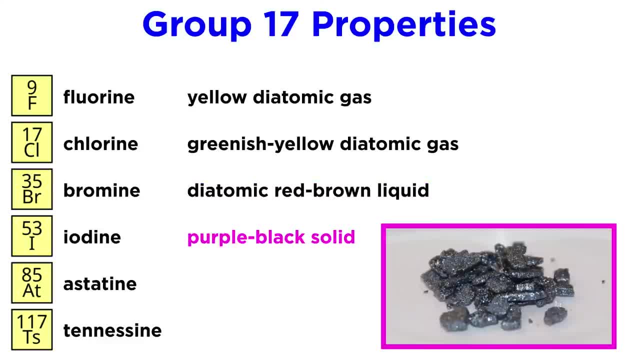 solid or gas at room temperature. And finally, iodine is a purple-black solid whose crystals easily sublime to generate a deep violet vapor. This is the only halogen with multiple allotropes, as, apart from the diatomic form, I3 minus, I5 minus, I7 minus and I9 minus are all possible. 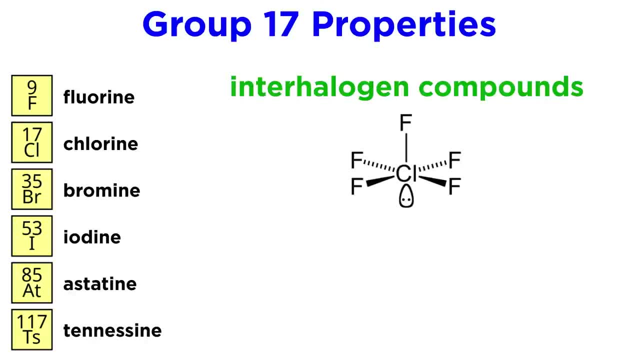 Another interesting feature of the halogens is their ability to form interhalogen compounds, Since nonmetals like to make covalent bonds with one another. this applies to the halogens and works well when the two halogens have very different electronegativities. 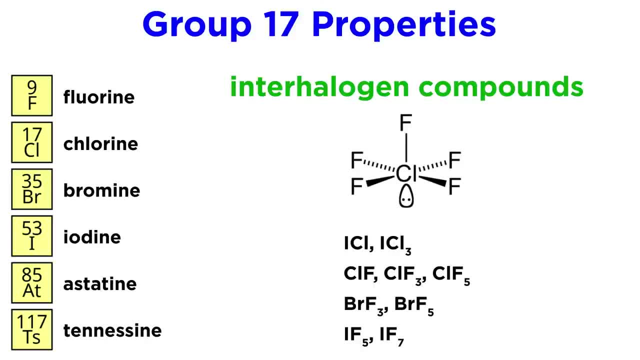 Here is a list of some common interhalogen compounds. Additionally, chlorine, bromine and iodine form many different oxyacids, such as the ones listed here, as well as the ones listed below, As the halides we are familiar with from organic chemistry. 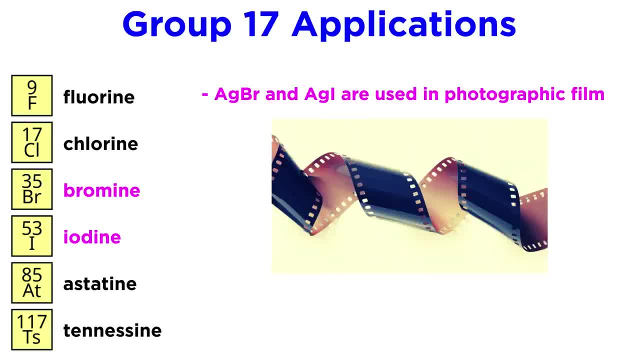 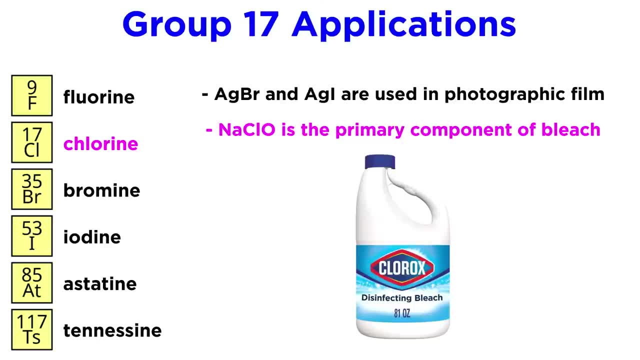 Moving on to applications, silver bromide and silver iodide are used in photographic film. Sodium hypochlorite is the primary component of bleach. Chlorine is also important for bleaching wood pulp and cotton cloth. Sodium chloride is table salt ubiquitous in cooking. 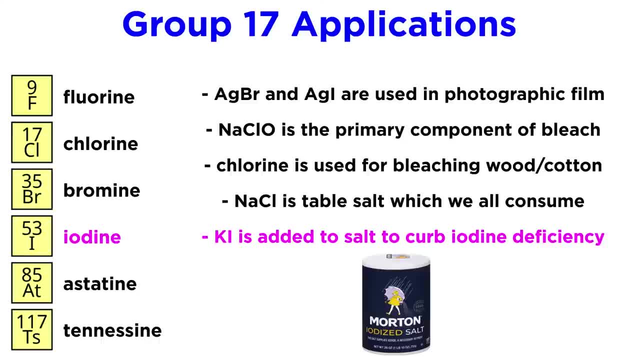 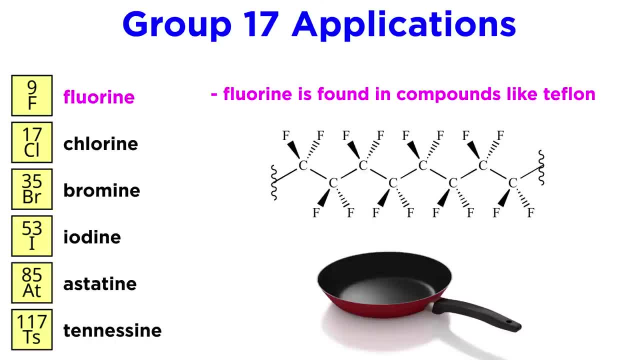 Potassium iodide is added to table salt in trace amounts to counter iodine iodine deficiency, which impacts thyroid function. Fluorine is found in interesting compounds like Teflon, which is useful in creating non-stick surfaces for a variety of products, and there are also many important fluorinated pharmaceuticals. 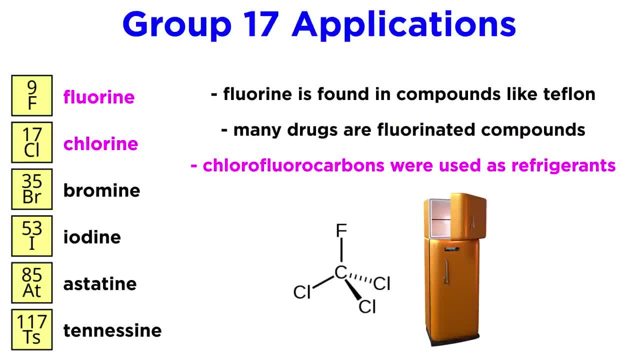 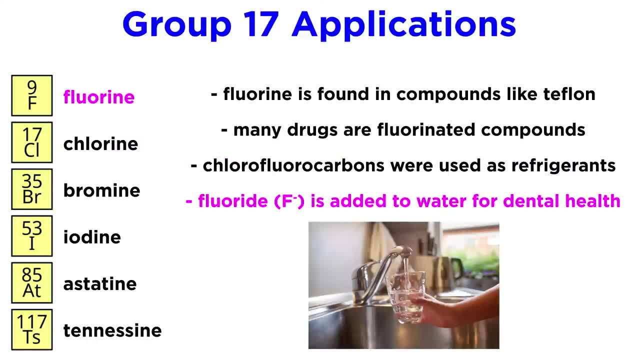 Chlorofluorocarbons, such as Freon, were used as non-toxic refrigerants, though this was eventually discontinued as it was discovered that these compounds were damaging the ozone layer. Fluoride, the anion of fluorine, is added to many public drinking water supplies to 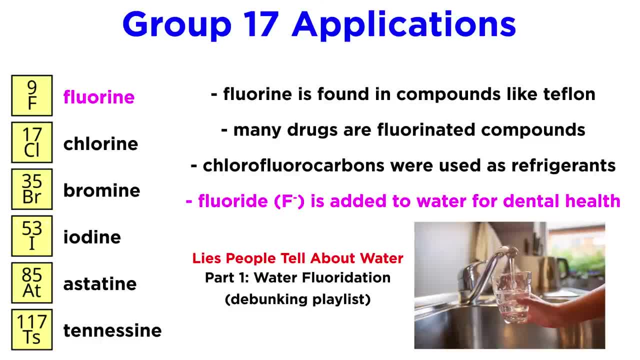 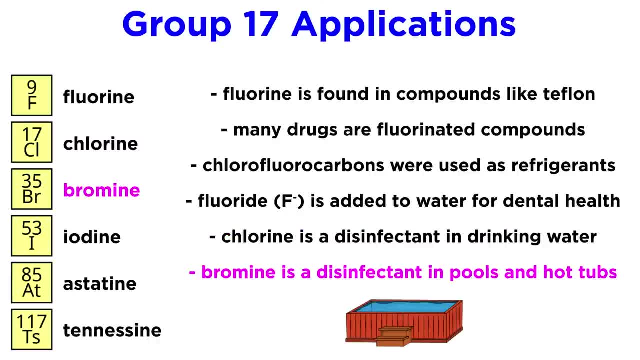 enhance dental health, as we discussed at great length in this video here. Chlorine is used as a disinfectant in community water supplies, while bromine is used as a disinfectant in hot water, like in hot tubs and some pools.